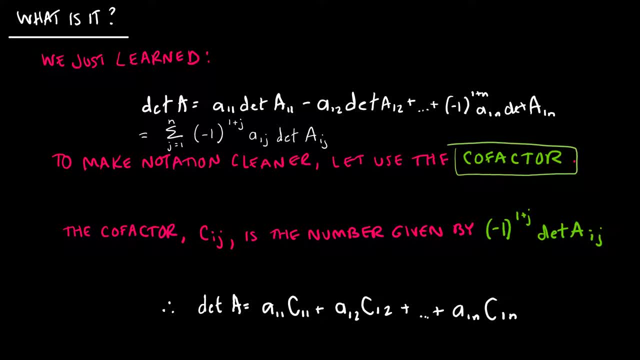 something called the cofactor, And we haven't talked about cofactor before and yet it's something that it's going to look very familiar to us. The cofactor, which we're going to denote Cij, is essentially going to take over the whole plus minus thing that we have going on. 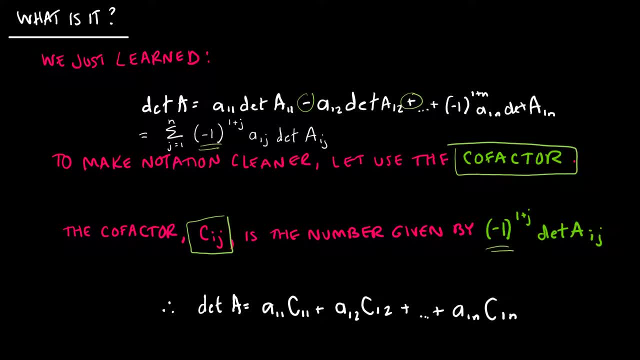 That's where that negative 1 comes in, just like it did here, And all of the determinant part of this. So it's going to essentially replace that part, And what we do is we take negative 1,- and this should be an i, not a 1,- negative 1 to the i plus. 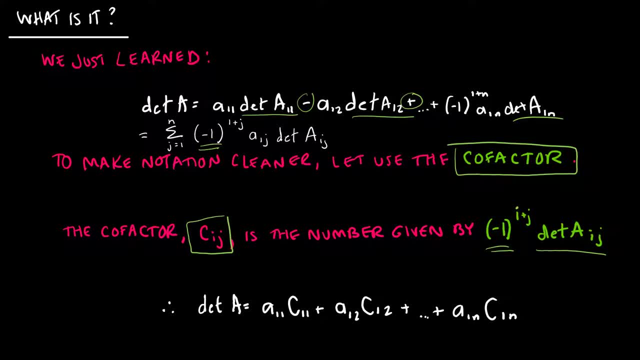 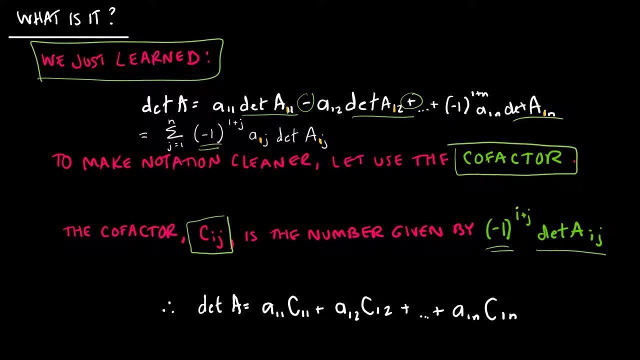 get the idea. We're only going across the first row. So what I'm telling you is, if we're using a cofactor, then I can go essentially across any row or any column, which we'll talk about on the next slide. So what this reduces to says that the 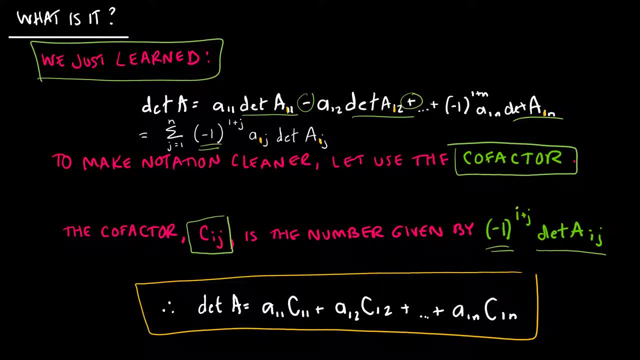 determinant of A is A11C11 plus A12C12 plus. Now why do I get to use pluses all of the time? Because now I have this negative 1 to the I plus J, which is going to give me that alternating 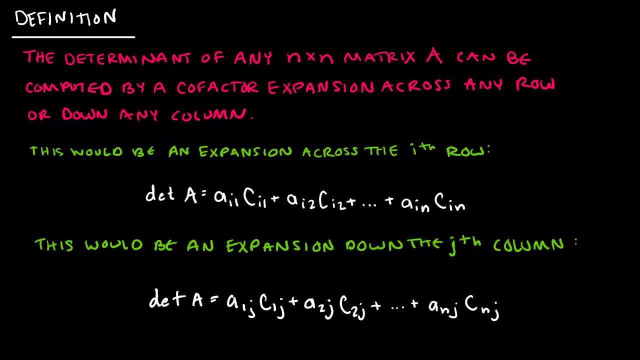 plus minus that I need. So now let's look at the definition. The determinant of any n by n, matrix A can be computed by a cofactor expansion across any row or down any column. So we can go across any row or any column. So previously we were just using the first row, every single time. 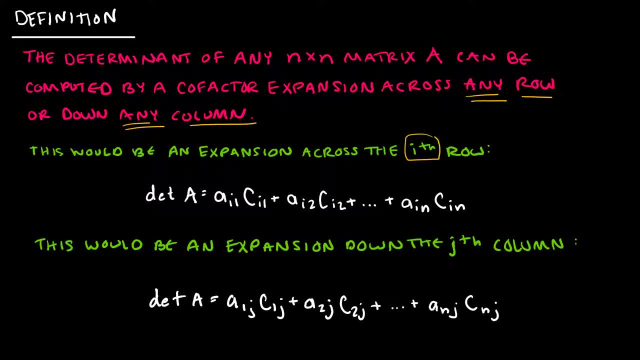 So, for instance, if I'm going across the ith row, which is what we just did before, except I was 1, so this was 1 and this was 1 and this was 1, but it doesn't have to be. 1 is essentially what we're. 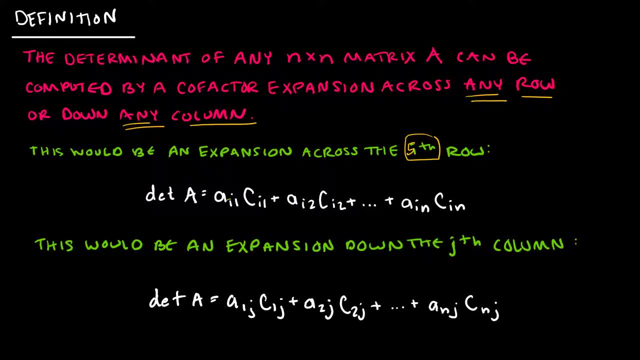 saying We can say across the fifth row. Well then it'd be 5, 1 and 5, 2.. Then you get the idea. So I can replace I with any row or I can go down any column, So it doesn't matter if I'm using a row or a column. So you might be asking: 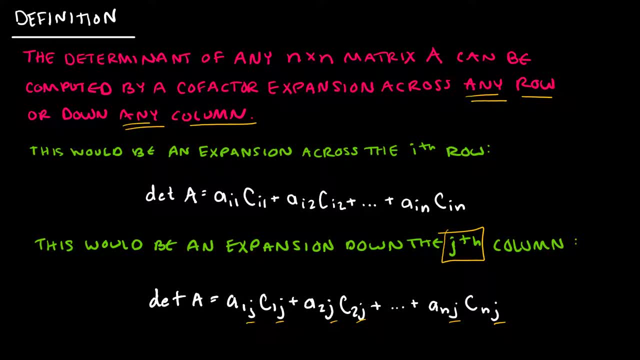 well, Professor Brame, why are you so geeked out about that? Well, because I don't like to do any extra work that I don't want to have to do. I'm kind of lazy. So if I get say a, 3 by 3,. 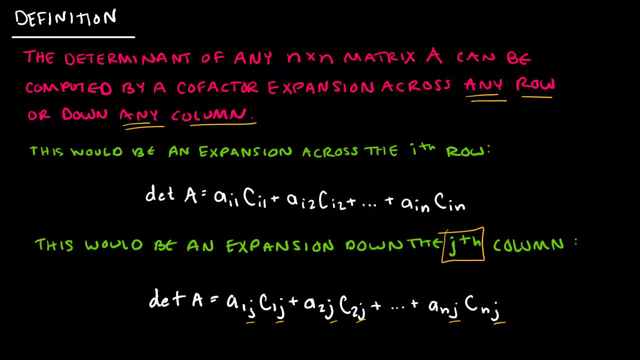 or a 4 by 4, or- God forbid- a 5 by 5 matrix, and I have to find the determinant. then I'm going to find the row or column that makes my work easier or easiest. Let's take a look Here. I have a. 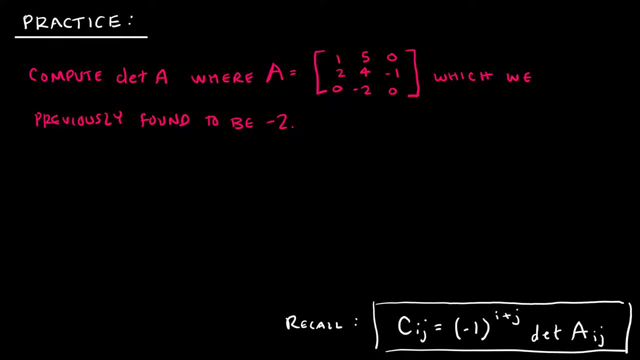 determinant A, and we already did this in our last video and we found that the determinant was negative 2.. Now, when we did this in our last video, we went across row 1, because that's all we knew how to do. But then I'm going to ask. 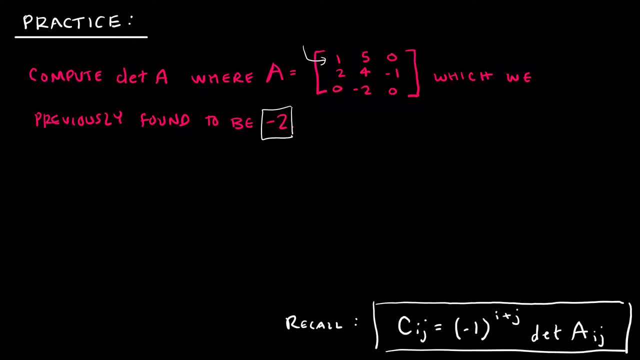 what makes my job the easiest. And what makes my job the easiest is as many zeros as I can get. So I might choose this column, which has two zeros, or I might choose this row, which also has two zeros, So choose one. I'm going to choose the row, since it's the last one I multiplied. 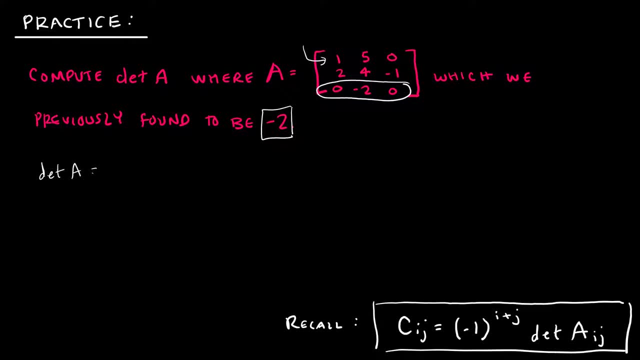 So to find the determinant of A remember, what I'm going to do is I'm going to take, and in this case I've chosen row 3.. So this is saying A 3, 1, and then C 3, 1, plus A 3, 2,, C 3, 2, plus A 3, 3,, C 3, 3.. 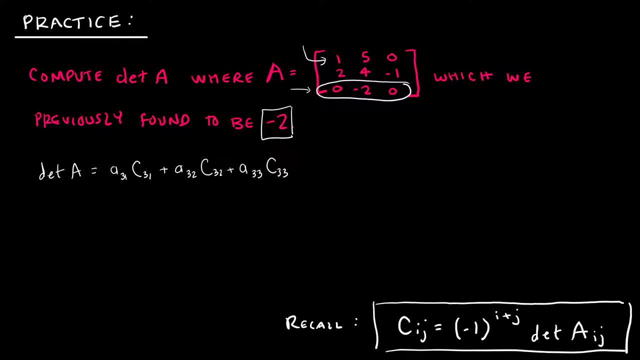 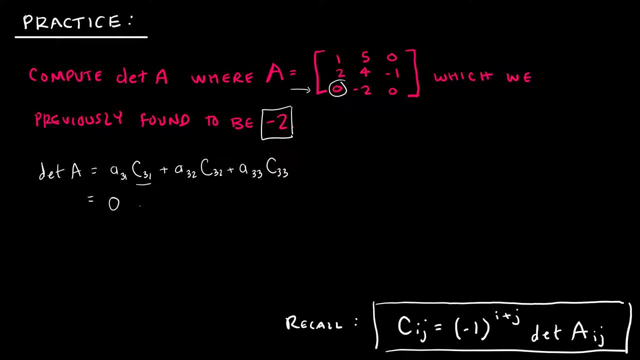 I don't care about C 3, 1, because I'm taking it times 0.. A 3, 2 is negative 2.. And then notice, I wrote this down here for you, in case you don't quite have it written down, or. 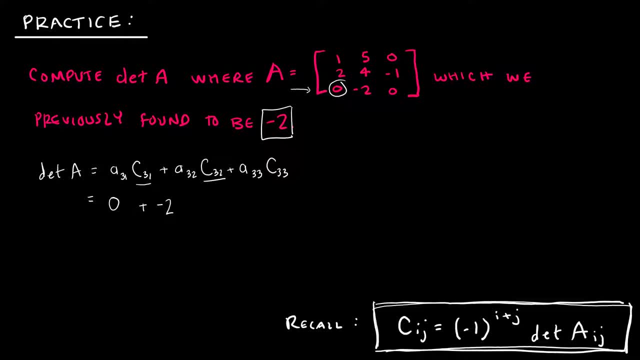 memorized. yet I need to take C 3, 2.. So C 3, 2 says take negative 1 to the I plus J, So that's 3 plus 2.. And then determinant. so instead of writing determinant, I'm going to use those straight brackets of A, 3, 2.. So again, 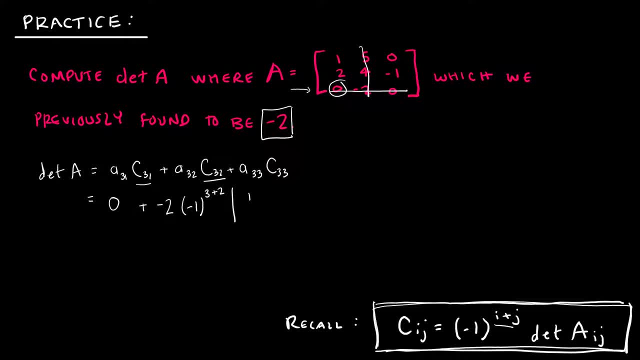 just like we did before. now I'm going to have 1,, 0,, 2, negative 1.. And then I'm going to take plus A 3, 3.. Oops, somehow switched to that one, Fat fingered that one, Switched to a new color. 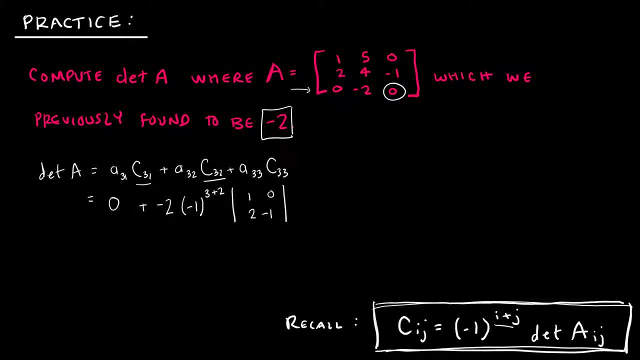 So now A 3, 2, or 3, 3 is 0. So it's plus 0. And I don't even care about this part then, because I'm taking it times 0.. So that's what I mean when I say I'm going to be smart and lazy is I'm going to try to get as many. 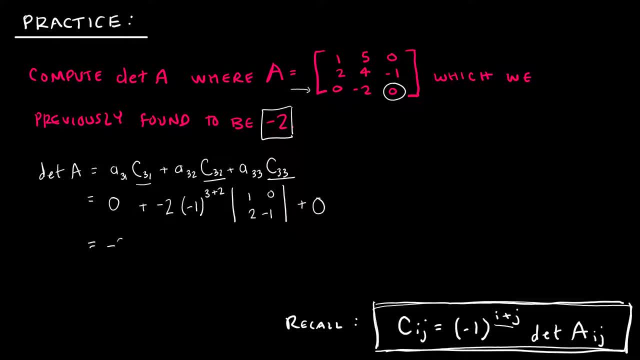 0s as possible, because now all I have to do I've got negative 2 and then I've got negative 1 to the 5th, which we know is negative 1.. And then I'm going to take that whoops times 1 times. 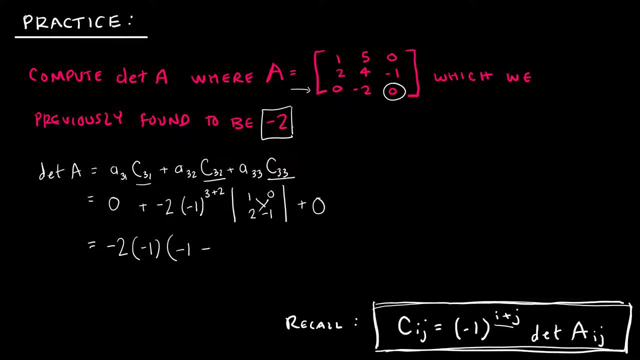 negative 1.. Minus 2 times 0. Oops, I almost wrote 2. That would be horrible. 2 times 0,, which is 0. So that gives me negative 2 times negative, 1 times negative 1, which gives me negative 2.. Now 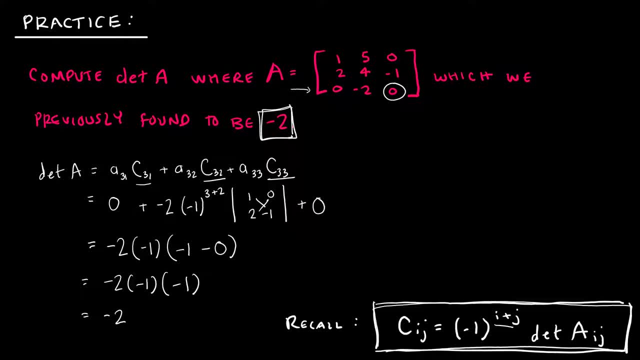 I had found that to be negative 2 before, but now I've just shown it again in a different way, using row 3 instead of row 1.. So just for fun, because I know you're having a blast, let's also do that again. So I'm going to take negative 1,, which is negative 1, times negative 1,. 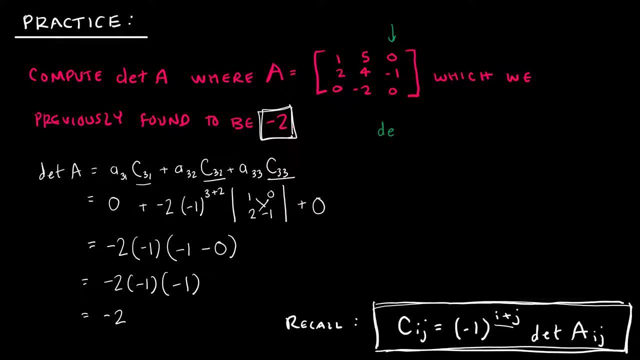 and do this for column 3.. So determinant A is going to be A13, C13, plus A23, C23, plus A33, C33.. So determinant A A13 is 0.. So again, I'm not going to worry about that. 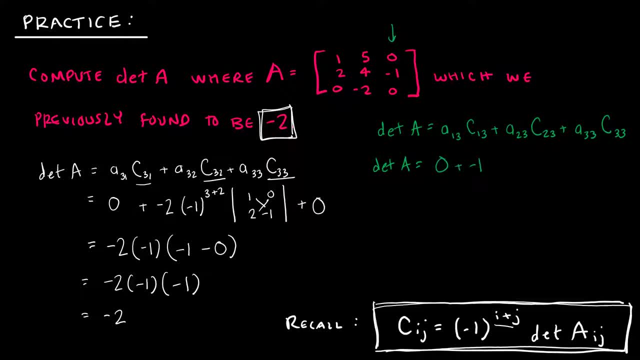 A23 is negative 1, because again second row, third column. And then I have to come down here, in case we haven't quite memorized it yet, and say now that's going to be negative 1 to the 2 plus 3.. And then the determinant of my matrix, 150 negative 2.. And then plus A33 is 0.. 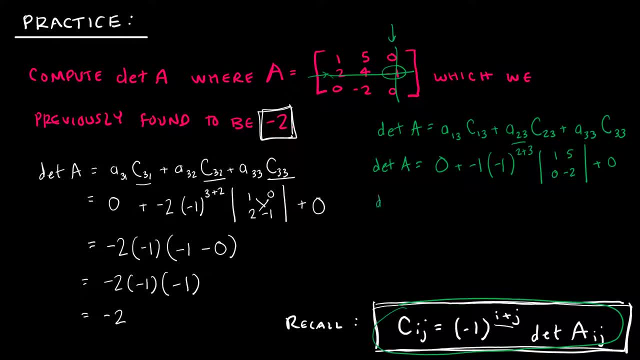 So again, I've done that, And then I'm going to take negative 1, which is negative 1, times negative 1, chosen one with a lot of zeros. so the determinant of A is going to be- we don't care about the 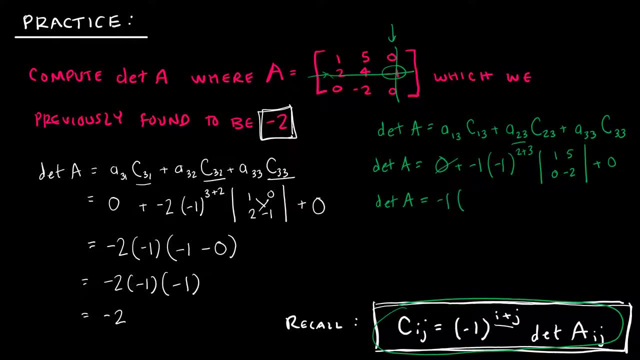 zero, negative 1, and then negative 1 to the 2 plus 3 is negative 1 to the 5th, which is negative 1.. Then I'm going to take 1 times negative 2 minus 0 times 5, and again we see negative. 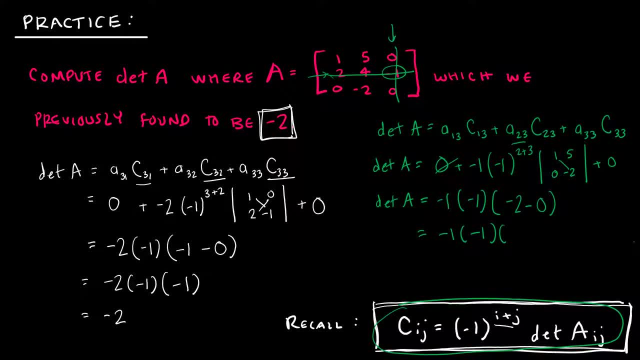 1 times negative, 1 times negative 2, which is negative 2.. So, again, a pretty easy way to do it, I'm going to go ahead and not write that 2 like that, and so I've confirmed it a couple of other ways. 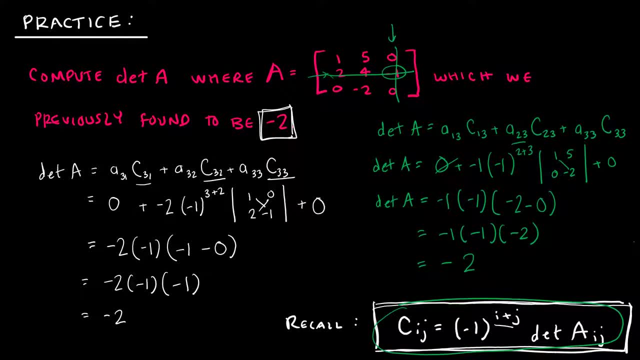 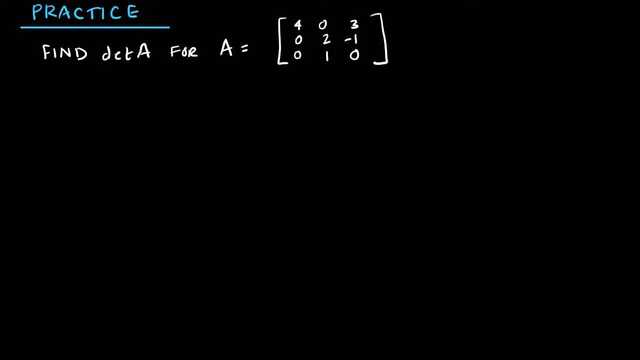 Now I could choose any row or any column, but again, be smart about it and choose a row or a column that has a lot of zeros. to make your life easier, Here's one for you to try: choose any row or column that you would like. 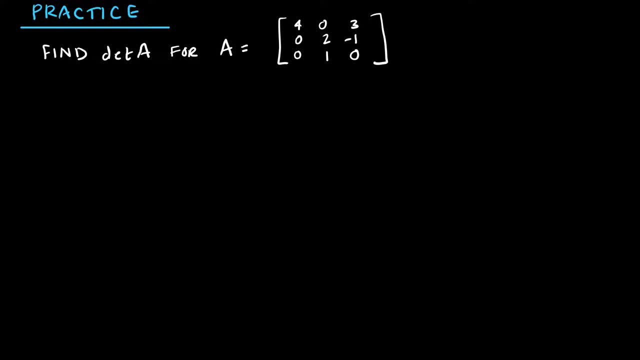 And find the determinant of A When you are ready. press play to see how you did So. I'm going to choose either row 1,- I'm sorry, column 1,- or row 3,, because both of those have two zeros and I just like to do as little work as possible. 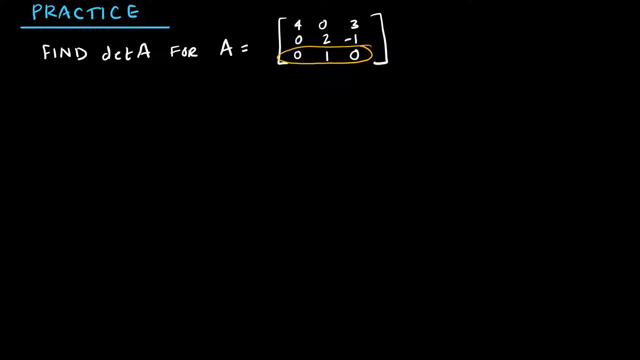 I'm actually going to choose row 3 here, and so that would give me: the determinant of A is equal to 0. 0 times. we don't care because it's a 0, plus 1 times negative 1 to the again this: 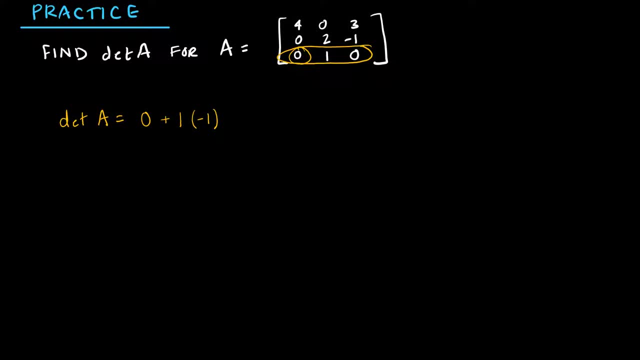 is row 3, column 2, so 3 plus 2, and then the determinant of 4,, 3, 0, negative 1, and then plus 0 times. we don't care. So that gives me. we're just going to disregard those zeros. 1 times negative 1 to the 5th. 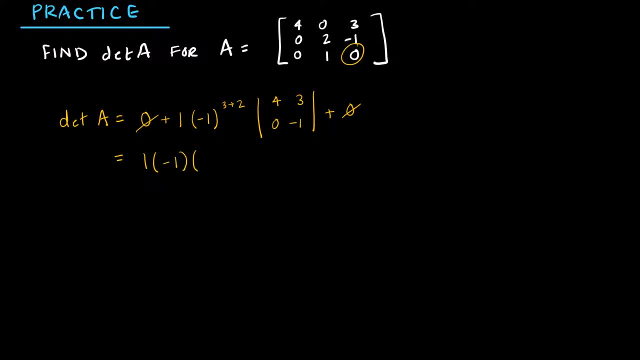 which is negative 1, times 4 times negative 1, minus 0 times 3,, which gives me 1 times negative, 1 times negative 4, which means my determinant is positive 4.. Now we're going to try to find the determinant of B. 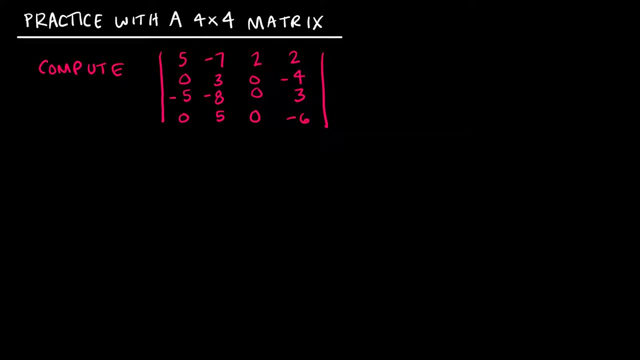 Now we're going to do a 4 by 4 matrix, which we haven't done before. Now, if you're feeling up to the challenge, please by all means go ahead and try this question on your own If you'd like. however, feel free to work through this one with me, since we've never 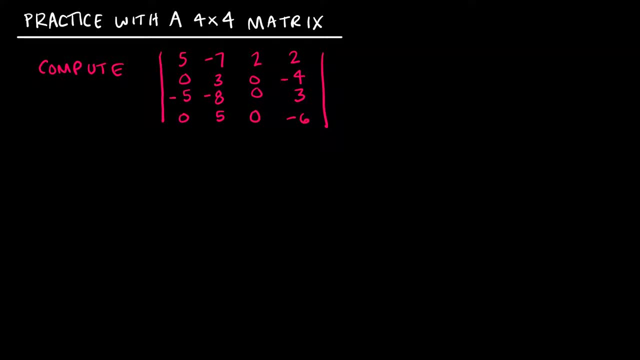 tried one like this before. So let's take a look. I need to find the determinant. So again notice: it doesn't say find the determinant, but it's given us these straight brackets, and those straight brackets indicate determinant. So when it says compute and then gives you the straight brackets, 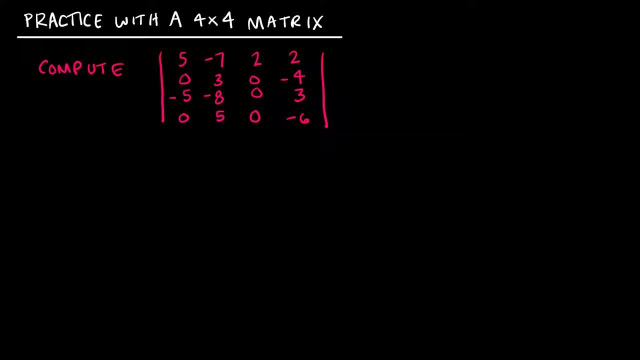 So when it says compute and then gives you the straight brackets and then gives you the straight brackets, it's the same as saying find determinant of A. So we'll just call it A for fun. So I'm going to find the determinant and I'm going to use this column because obviously 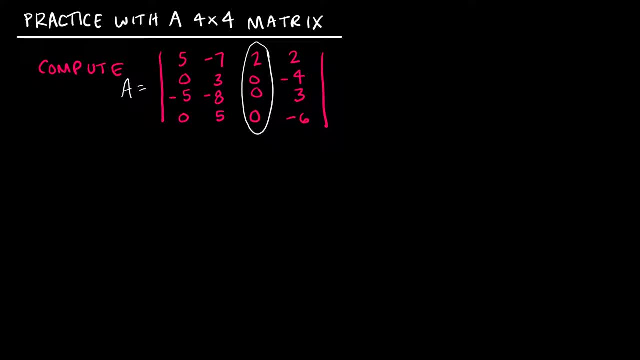 it's got a lot of zeros in it and I want to do as little work as possible, So the determinant of A is going to be 2 times negative 1 to the. this is first row, third column, 1 plus 3.. 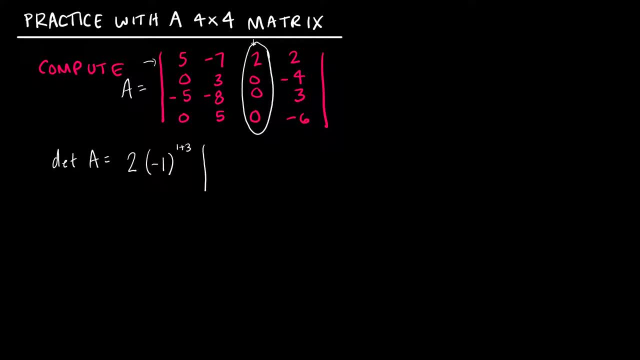 And then I'm finding the determinant of what's left over, which is 0, 3, negative 4, negative 5, negative 8, 3, 0, 5, negative 6.. And then we can see that, as I work my way down the column, that would be plus 0, plus. 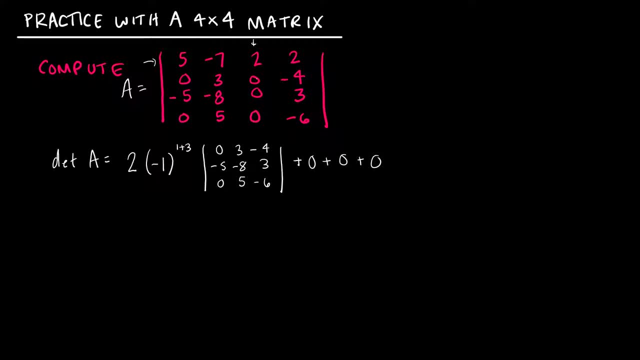 0, plus 0. And we don't care about what the new matrices would be, because we're going to multiply them by 0 anyway. So that's where we are right now. Now, negative 1 to the 1 plus 3 is negative, 1 to the 4th, which is positive 1.. 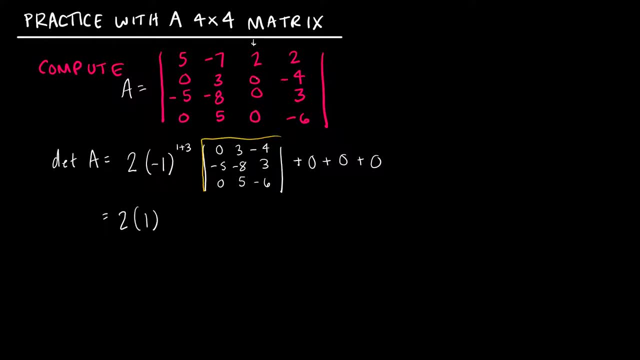 And then I need to now find the determinant of this. So how do I find the determinant of a 3 by 3?? Well, lucky us, we already know how to do that. We're going to choose a row or column, and I'm choosing this column. 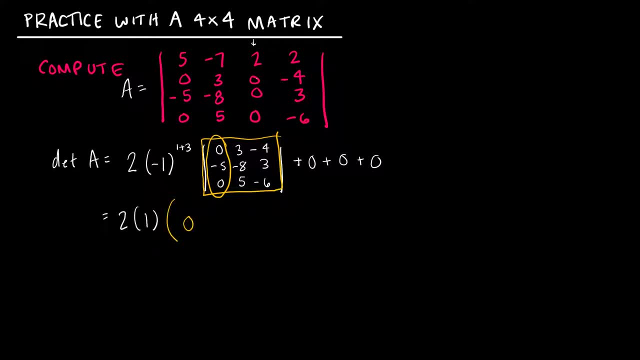 And that's going to tell me to take 0 times what's left over, which I don't care about, that, Plus negative 5 times negative 1 to the. that's second row, first column, And then the determinant of what's left over, which is 3, negative 4, 5, negative 6.. 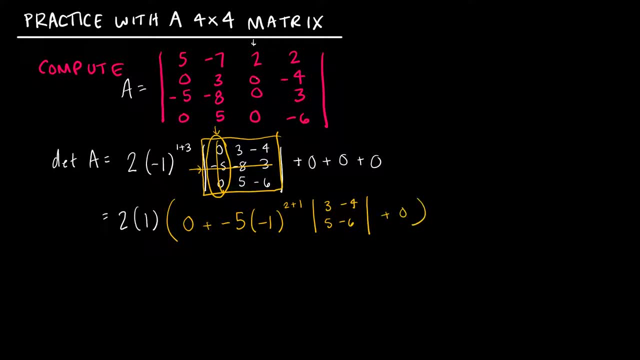 And then, of course, plus 0. So I still have my 2 times 1, which is 2 on the outside and on the inside. I'm going to not worry about the 0. I have negative 5 times negative: 1 to the 3rd, which of course is negative 1.. 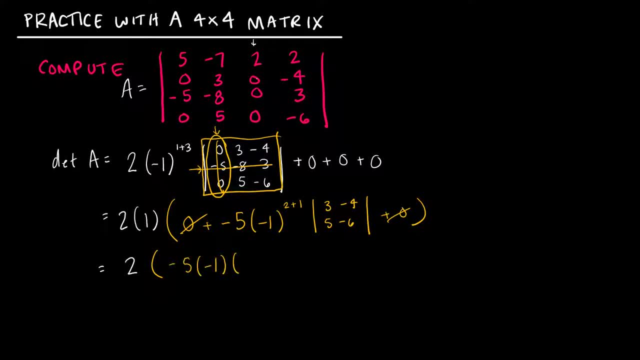 So negative 5, negative 1, and then negative 18 minus negative 20.. So I'm going to keep that 2 on the outside for now. I've got negative 5 times negative 1,, which is positive 5, and then I have negative 18. 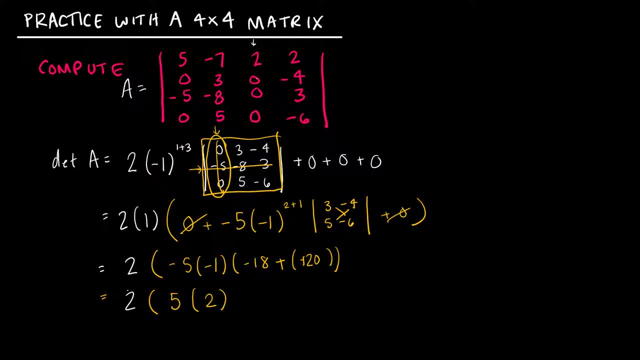 plus 20.. Which is 2.. And then, if I multiply this, I get 2 times 5,- I think I forgot a parenthesis- 2 times 5 times 2, which is 20.. So my determinant is in fact 20.. 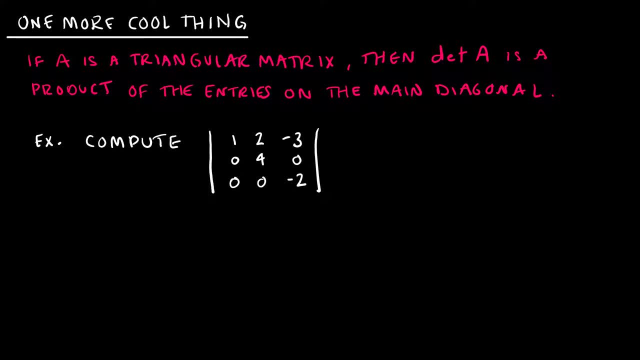 Let's look at just one more cool theorem, And I'm not going to go through a proof for this theorem, but I'm just going to show you an example that it does in fact work Before I talk about what's in pink. 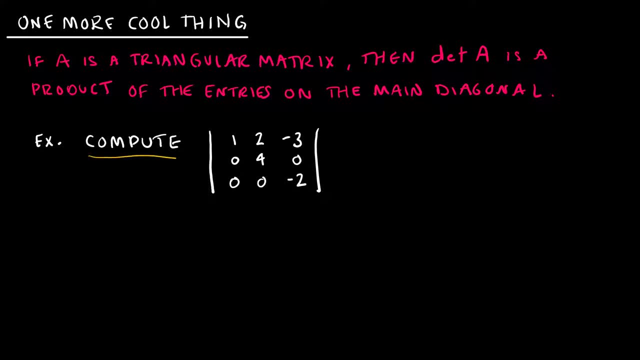 Let's just go ahead and compute, based on the way that we just learned how to do it. Let's compute the determinant of this matrix. If I were finding the determinant, I would choose probably this row right here. So the determinant of A would be 0 plus 0 plus negative 2, and then I would take negative. 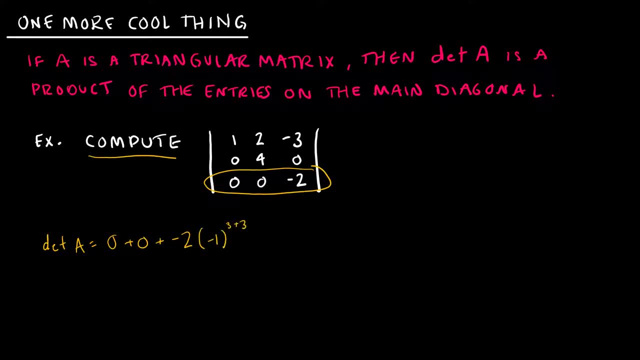 1 to the 3 plus 3, and then the determinant of 1 to 0.. So I'm going to put the 0's And it's not necessary for you to put the 0's. I put the 0 because the first term is 0 and the second term is 0.. 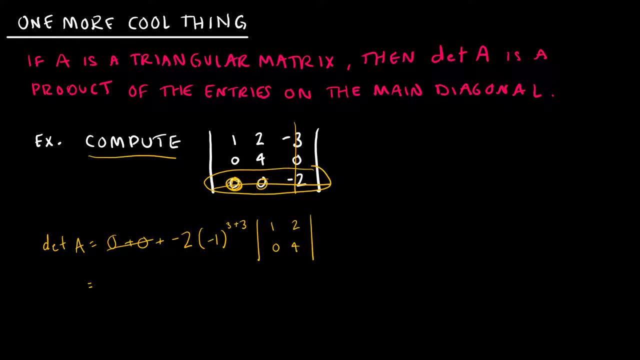 But it's just fine to omit those. So I have negative 2 and then negative 1 to the 6,, which is positive 1.. And then I'm going to take 1 times 4,, which is 4, minus 0 times 2.. 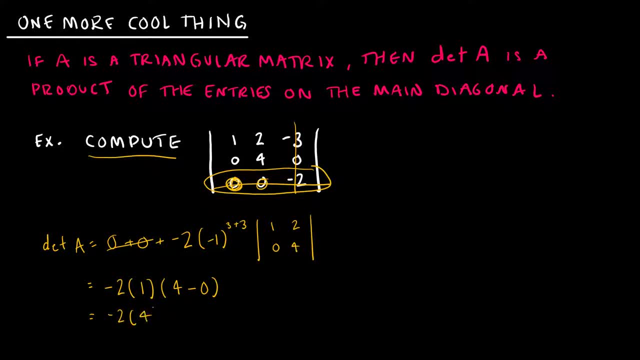 And that gives me negative 2 times 4, which is negative 8.. So what this theorem does, Which is theorem 2 in your textbook, What this theorem says is, if you have a triangular matrix, which we know a triangular matrix- I'm not talking about reduced row echelon form, but I am. 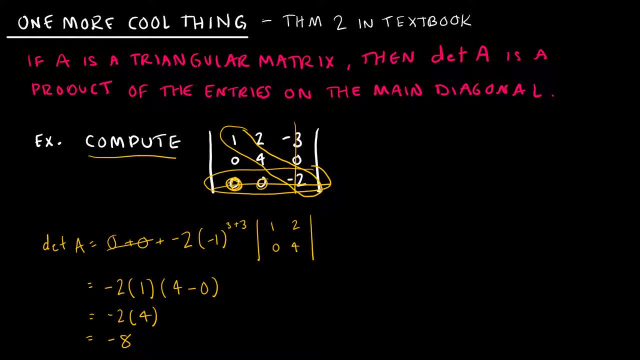 talking about anything essentially below that diagonal has to be 0's, And I of course do have a triangular matrix here. This theorem says: if A is a triangular matrix, then the determinant of A is a product of the integral matrix. I can find the determinant of A by taking 1 times 4 times negative, 2.. 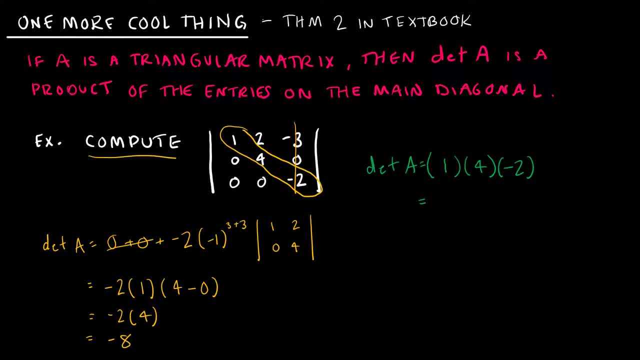 So just multiply those values in the diagonal, which is negative 8.. And we just found that it was in fact negative 8.. So again, that is not a proof. This is just an example that it works. I'm sure that you can find a proof. 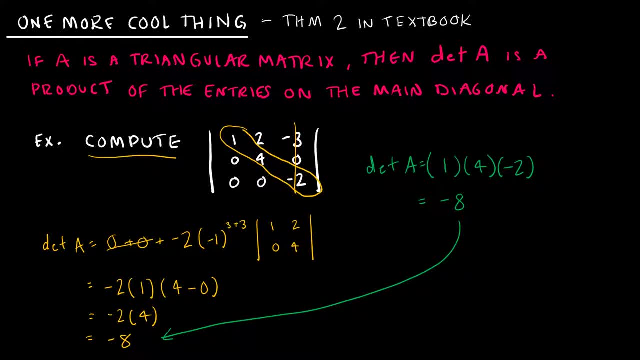 Your textbook does not have a proof, but I'm sure you can find a proof if you Googled. I'm not going to go through that with you.